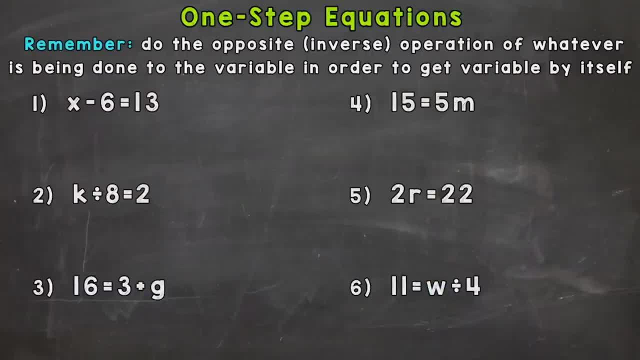 In this video, we're going to discuss how to solve one-step equations. And as you can see, there are six problems on your screen that we're going to go through in order to get this down. Now, up top, I have a hint we need to remember as we go through these problems. So we're going to do the opposite, or inverse, operation of whatever is being done to the variable in order to get the variable by itself. Now, that may not make any sense at first, but as we go through these problems, you'll start to see what I mean by that. Again, main goal is getting the variable by itself. And just to reiterate, inverse means opposite. It means to do the opposite. 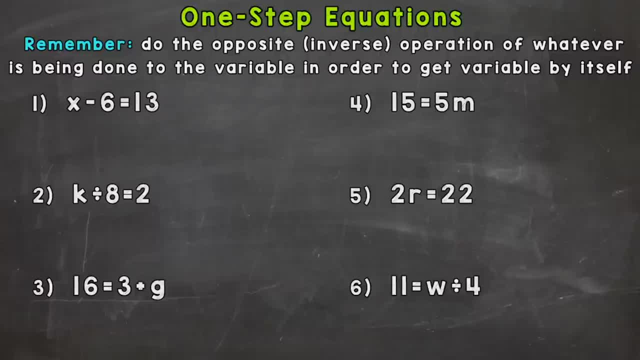 So addition, the inverse, would be subtraction. Multiplication, the inverse, would be division. 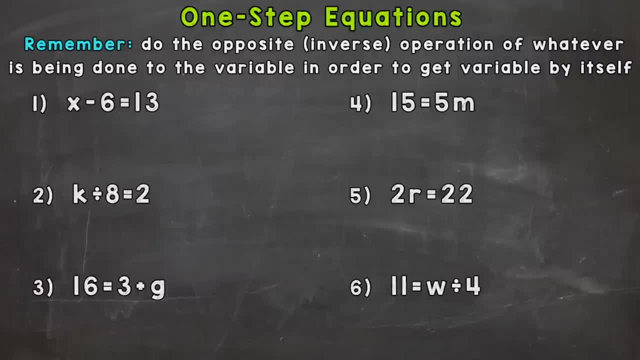 So let's jump right into number one here and see how we solve one-step equations. So for number one, we have x minus 6. So we need to take a look at what we're doing to the variable x, our missing piece. And we're subtracting 6. So we need to do the opposite. So that would be adding 6. So we need to add 6 to that side. 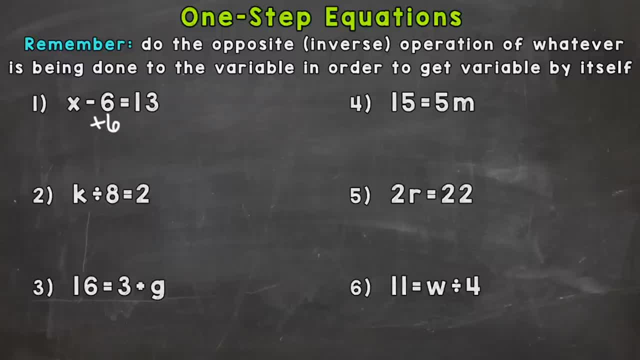 And the reason we do that, because we have x minus 6 plus 6, the minus 6 plus the 6 gives us 0, essentially cancelling those 6s out. So we're just left with the x that gives us the x by itself. 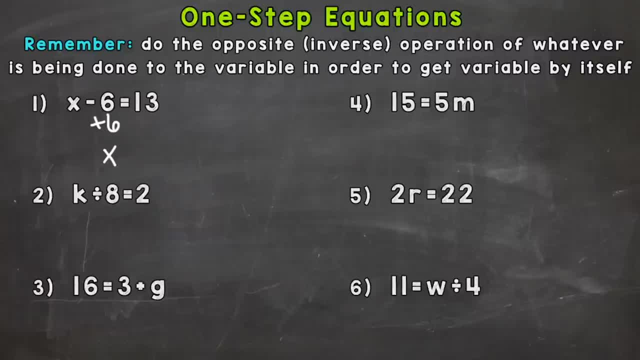 Now, in order to keep that equation balanced, we have to do the same thing over and over again. So we're going to do the same thing over and over again. So we're going to do the same thing over and over again. So we're going to do the same thing to both sides. Whatever you do to one side, you have to do to the other. So we added 6 to the left, so we need to add 6 to the right. 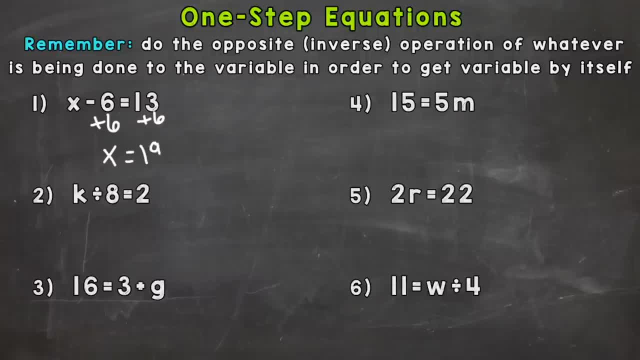 So 13 plus 6 gives us 19. 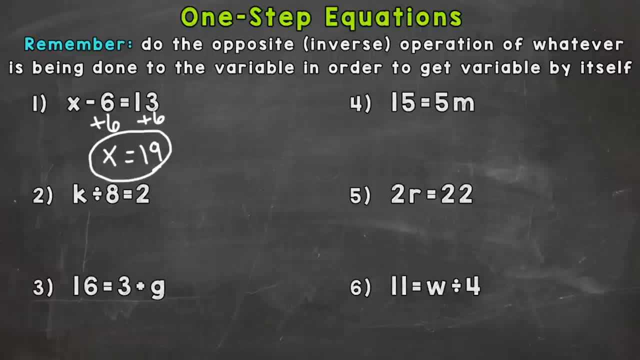 So x equals 19. And we always double check to see if this makes sense and our answer for the variable is correct. 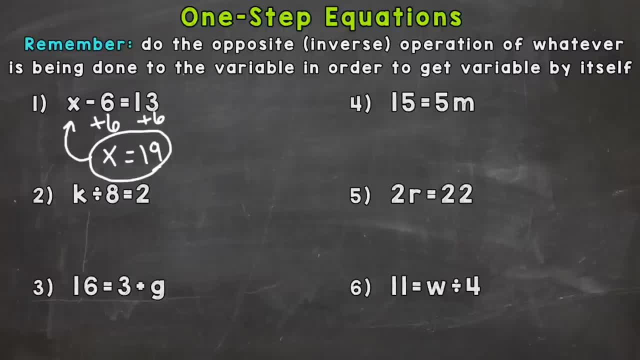 So let's plug in 19 for our x here. 19 minus 6. 19 minus 6 equals 13, and that is true. It is correct. 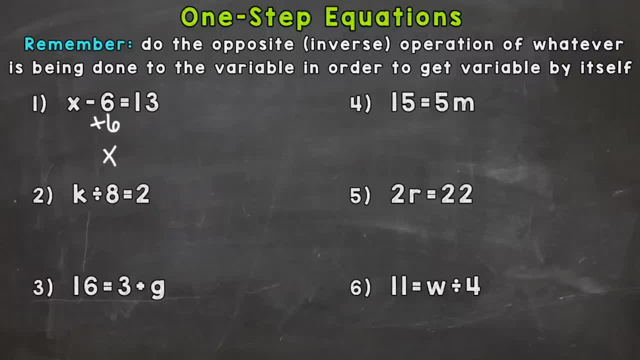 Now, in order to keep that equation balanced, we have to do the same thing over and over again. So we're going to do the same thing over and over again. So we're going to do the same thing over and over again. So we're going to do the same thing to both sides. 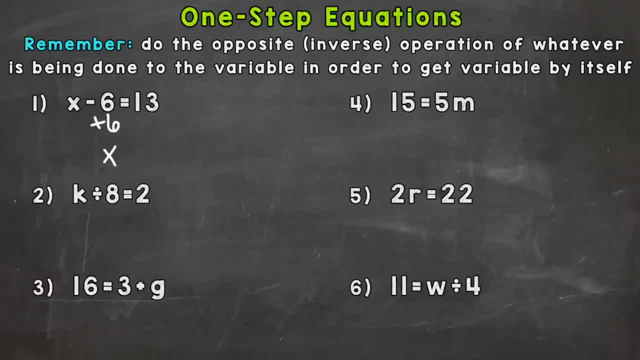 Whatever you do to one side, you have to do to the other. So we added 6 to the left. so we need to add 6 to the right. So 13 plus 6 gives us 19.. So x equals 19.. 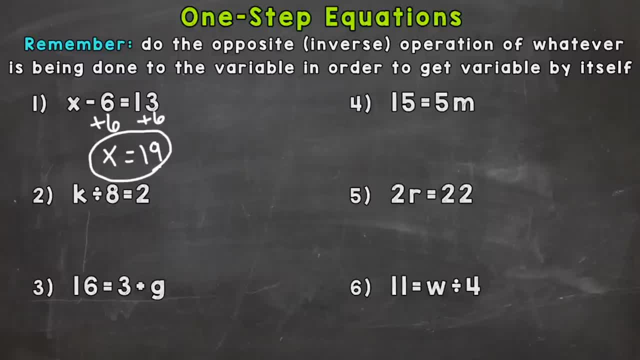 And we always double check to see if this makes sense and our answer for the variable is correct. So let's plug in 19 for our x here, 19 minus 6.. 19 minus 6 equals 13,, and that is true. 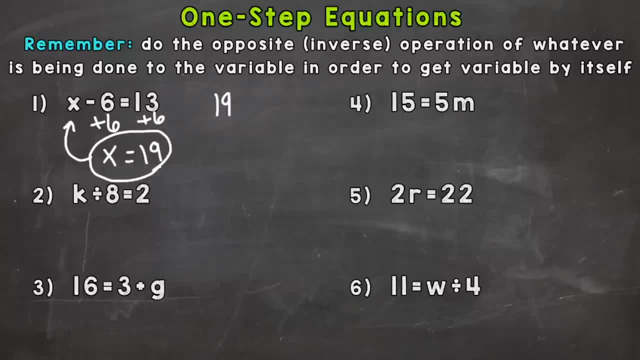 It is correct. I'm even going to come to the side here. plug it in: 19 minus 6 equals 13.. That is true, So we're good to go. We have the correct answer for what x equals. Let's take a look at number two. 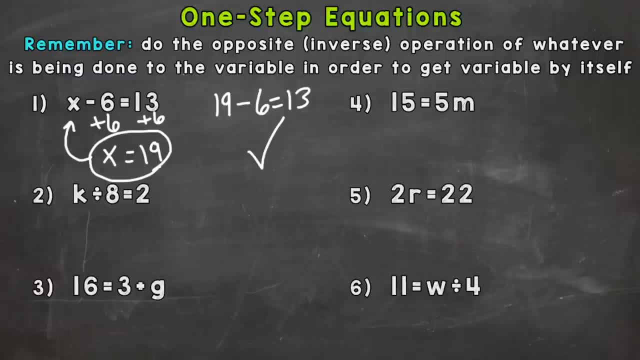 We have k, divided by 8, equals 2.. We have k divided by 8, equals 2.. So what are we doing to the variable? Well, we're dividing by 8.. So we need to do the opposite to that side to get rid of the dividing 8.. 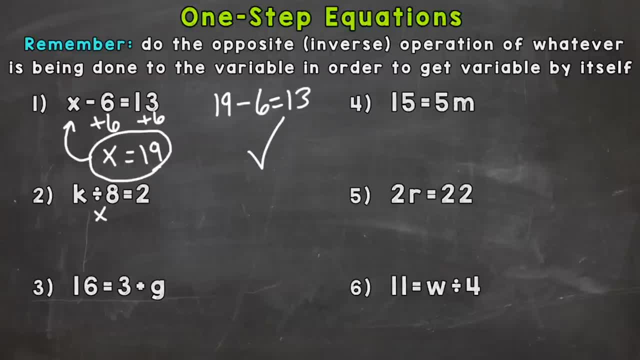 So we need to multiply by 8.. k divided by 8 times 8,, well those 8s would equal 0 or cancel out. So k is by itself. But whatever we do to one side, we have to do to the other to keep everything balanced. 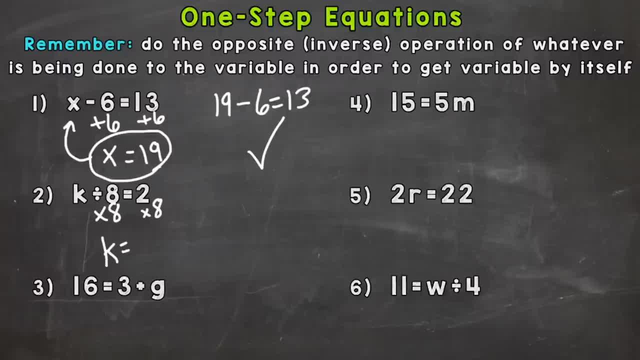 So we get to the point where k is by itself k equals. well, 2 times 8 is 16.. k equals 16.. Let's see if that's true. Let's plug in 16 for k. 16 divided by 8 equals 2.. 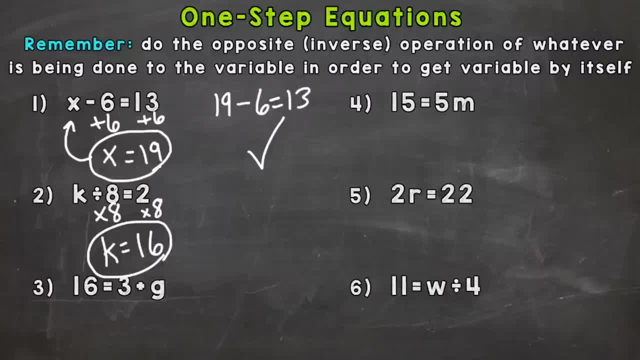 So k indeed does equal 16.. Let's take a look at number three. Now here we have the answer on the left hand side and our variable on the right. That's okay, That's fine. That happens in algebra sometimes. So we're adding 3 to g. 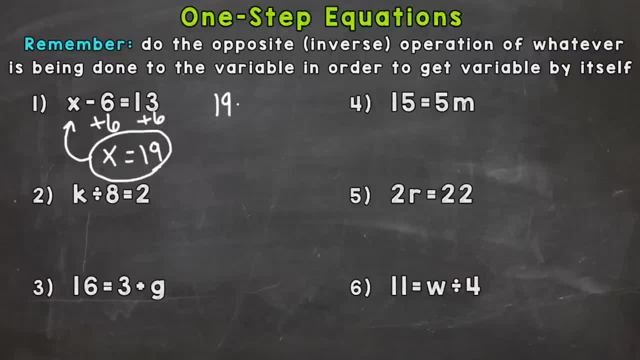 I'm even going to come to the side here, plug it in. 19 minus 6 equals 13. That is true. So we're good to go. 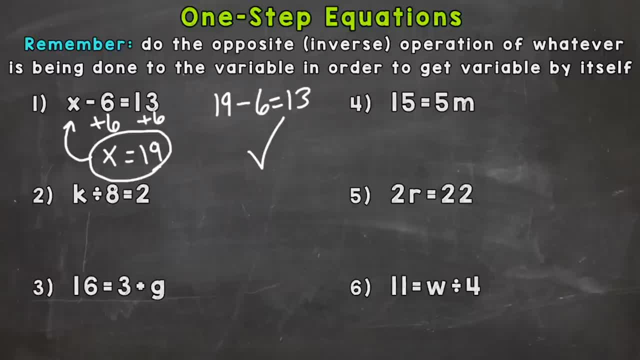 We have the correct answer for what x equals. Let's take a look at number two. 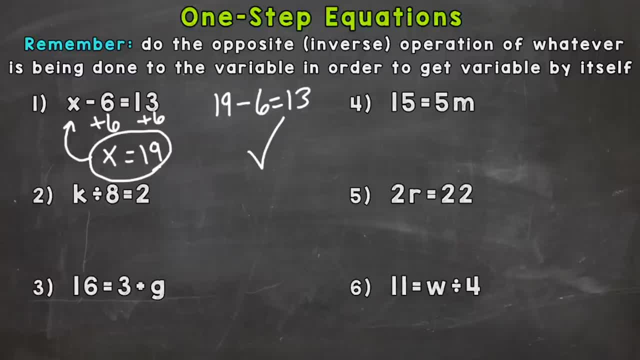 We have k divided by 8 equals 2. We have k divided by 8 equals 2. So what are we doing to the variable? Well, we're dividing by 8. 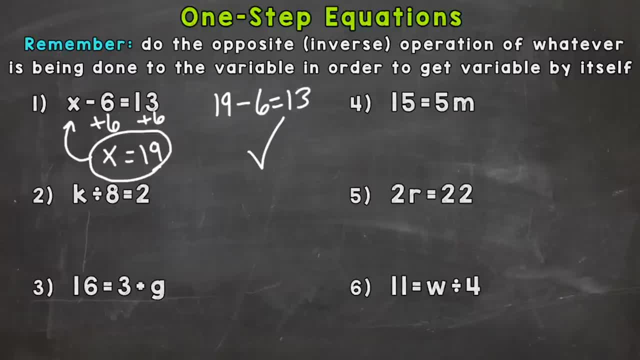 So we need to do the opposite to that side to get rid of the dividing 8. 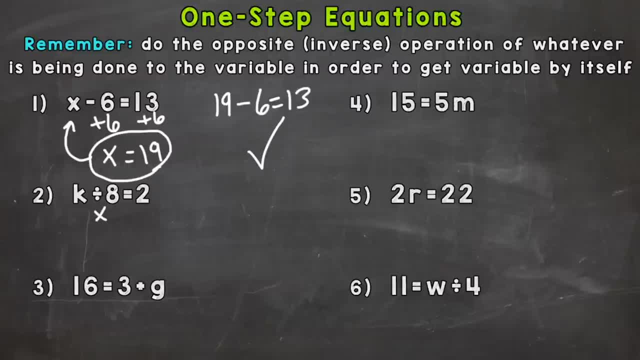 So we need to multiply by 8. k divided by 8 times 8, well, those 8s would equal 0 or cancel out. So k is by itself. But whatever we do to one side, we have to do to the other to keep everything balanced. So we get to the point where k is by itself. k equals, well, 2 times 8 is 16. k equals 16. 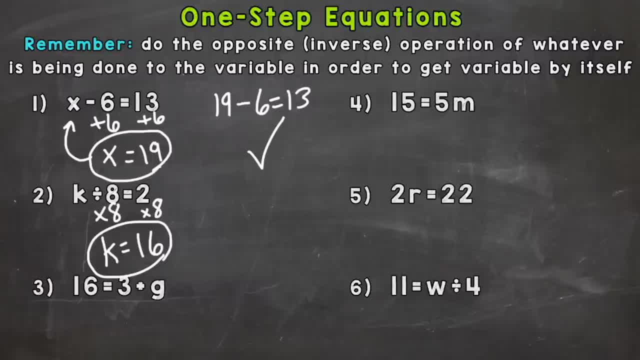 Let's see if that's true. Let's plug in 16 for k. 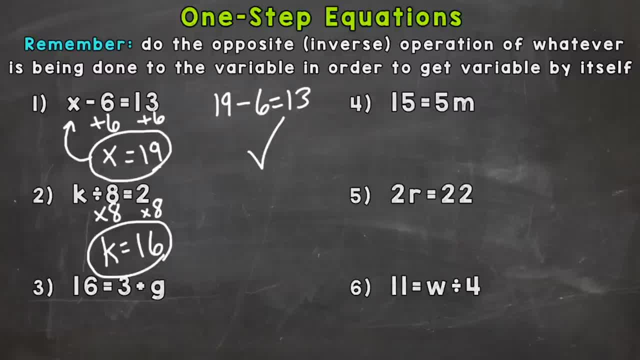 16 divided by 8 equals 2. So k indeed does equal 16. 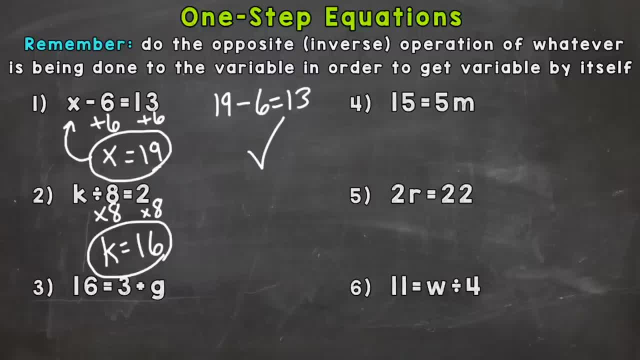 Let's take a look at number three. Now here we have the answer on the left-hand side and our variable on the right. That's okay. 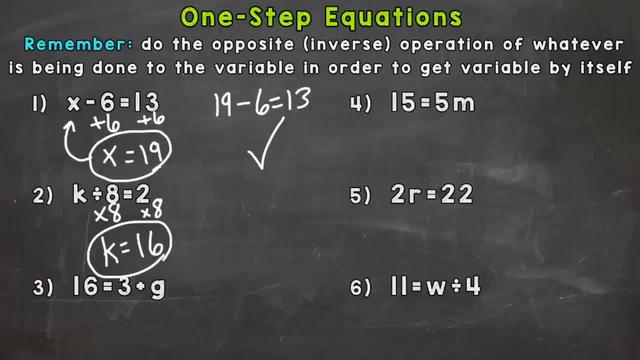 That happens in algebra sometimes. So we're adding 3 to g. So we need to do the opposite to that side to get g by itself. So we need to subtract 3. 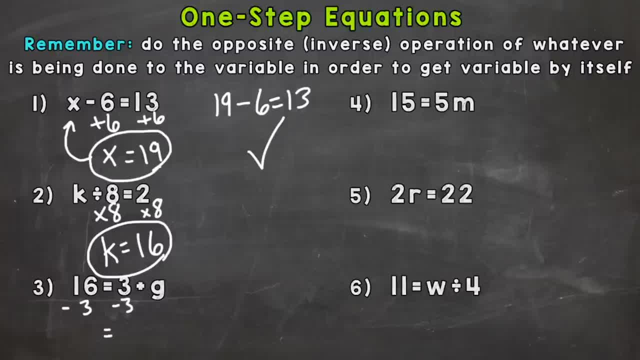 And we need to do it to both sides. So we get g equals 13. And I always like to rewrite with the variable first, g equals 13. And let's double check. 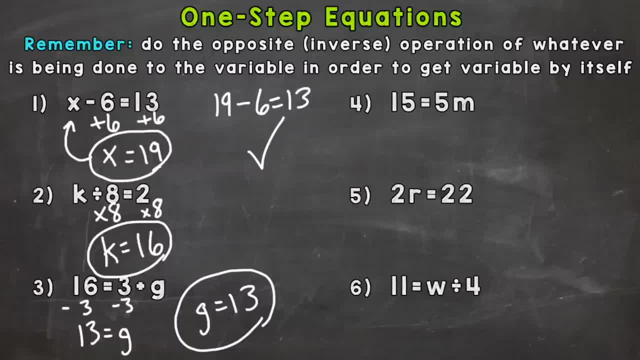 Does 3 plus 13 equals 16? Yes. So we have the correct answer for the variable. 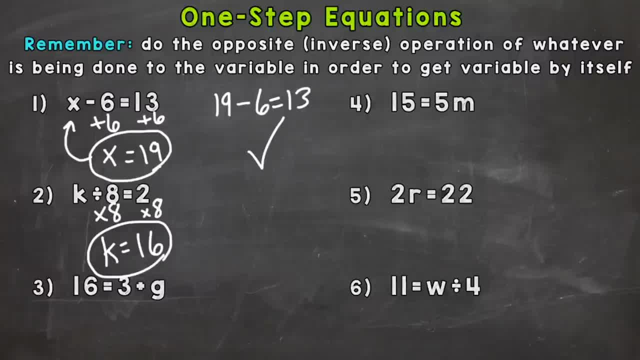 So we need to do the opposite to that side to get g by itself. So we need to subtract 3, and we need to do it to both sides, So we get g equals 13.. And I always like to rewrite with the variable first: g equals 13.. 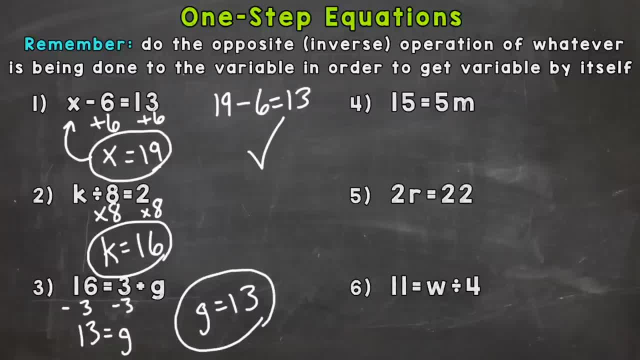 And let's double check: Does 3 plus 13 equals 16?? Yes, so we have the correct answer for the variable Number 4, we have 15 equals 5m. Now, a number right next to a variable or a letter means multiplication. 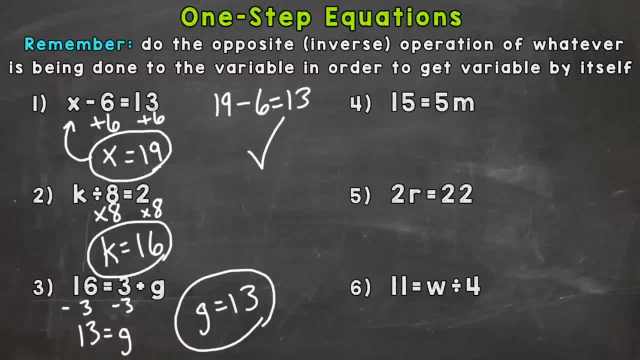 So we're multiplying by 5 here. So the opposite of multiplying by 5 would be dividing by 5.. That would give us our m by itself. And I put it in fractional form, and fractions are division here That means divide by 5.. 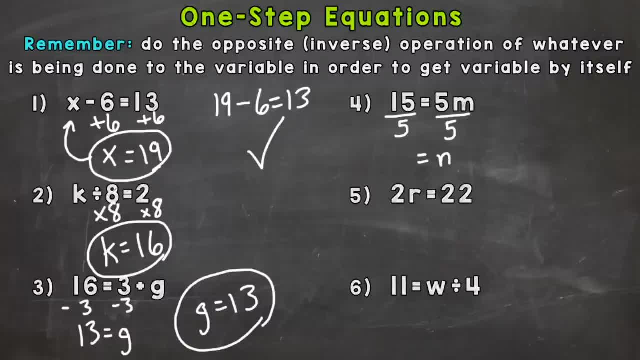 So do it to both sides, So we have the m by itself, and then 15 divided by 5 gives us 3.. So m equals 3.. Let's double check: 5 times 3 does equal 15.. So we have the correct answer there. 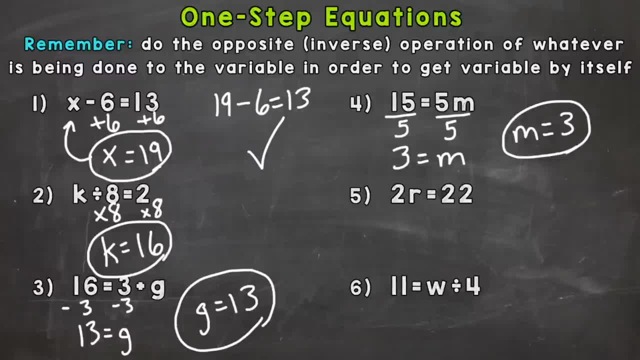 Number 5, we have 2r equals 15.. Number 6, we have 2r equals 22. So we're multiplying by 2.. Again, number next to a letter means multiplication, So we need to divide both sides by 2.. 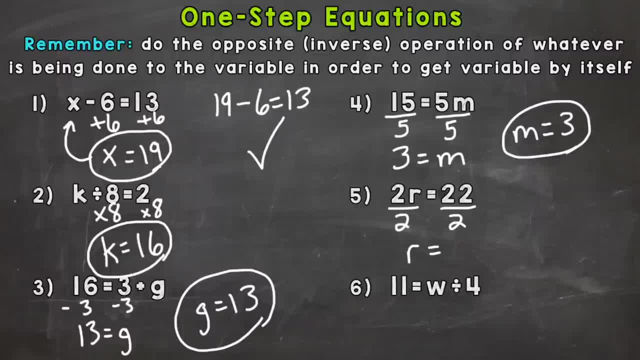 That gives us r by itself, and 22 divided by 2 equals 11.. So r equals 11.. Let's double check: 2 times 11 does equal 22,. so we're good to go there. Number 6,: 11 equals w divided by 4.. 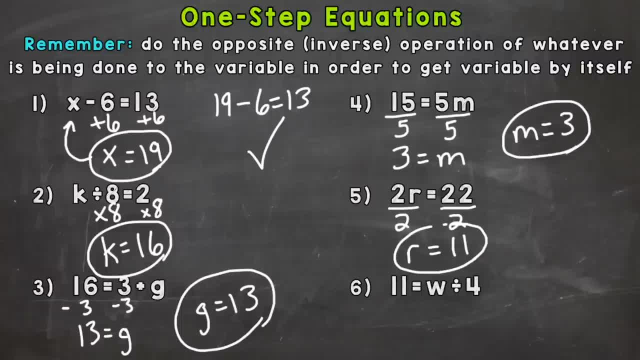 So we're dividing by 4.. The opposite would be multiplying by 4.. So let's multiply by 4 to get w by itself, And then, whatever we do to one side, we need to do to the other in order to keep everything balanced. 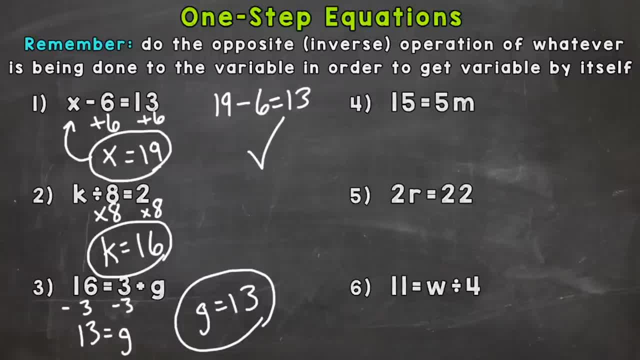 Number four. We have 15 equals 5m. 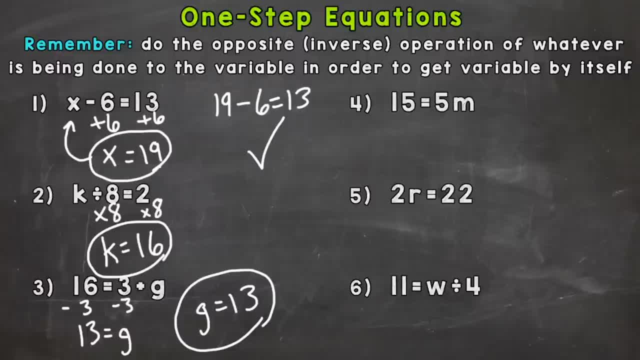 Now a number right next to a variable or a letter means multiplication. So we're multiplying by 5 here. So the opposite of multiplying by 5 would be dividing by 5. That would give us our m by itself. And then I put it in. I put it in fractional form, and fractions are division here. That means divide by 5. So do it to both sides. So we have the m by itself. 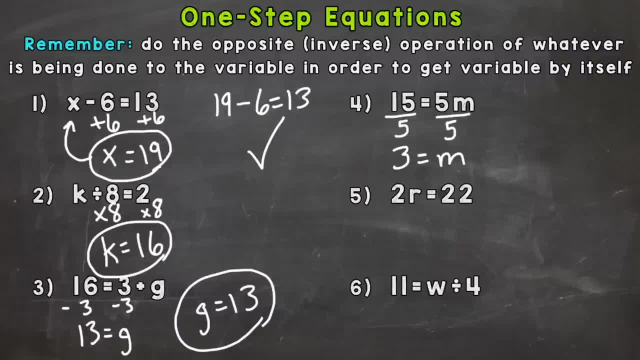 And then 15 divided by 5 gives us 3. So m equals 3. Let's double check. 5 times 3 does equal 15. So we have the correct answer there. 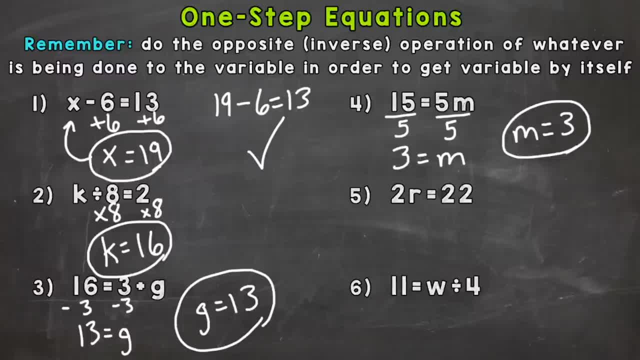 Number five. We have 2r equals 22. That's correct. 2. 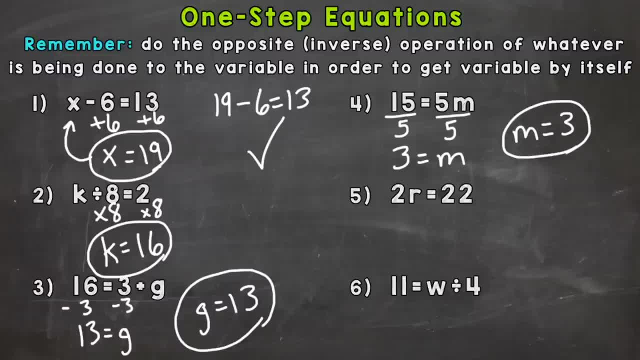 So we're multiplying by 2. Again, number next to a letter means multiplication. So we need to divide both sides by 2. That gives us r by itself. And 22 divided by 2 equals 11. So r equals 11. 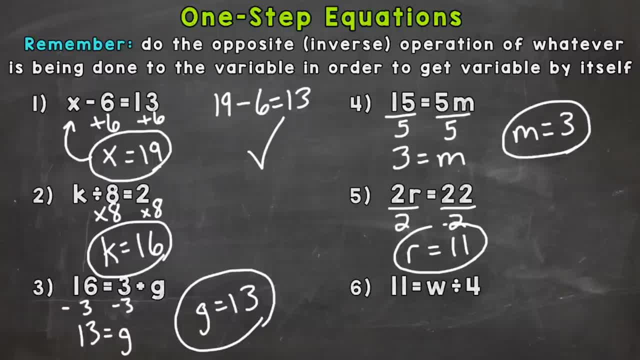 Let's double check. 2 times 11 does equal 22. So we're good to go there. Number six. 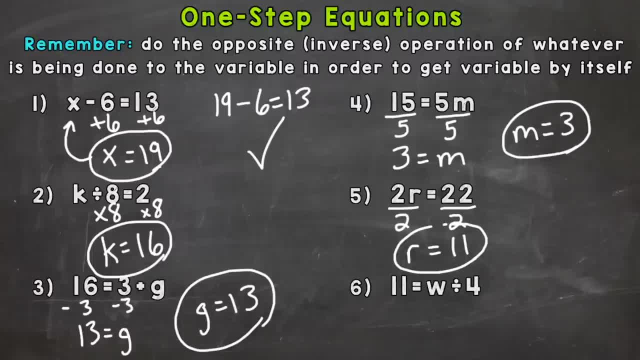 11 equals w divided by 4. So we're dividing by 4. The opposite would be multiplying by 4. So let's multiply by 4 to get w by itself. And then whatever we do to one side, we need to do to the other in order to keep everything balanced. So we end up with an answer of 44 for the value of w. So w equals 44. 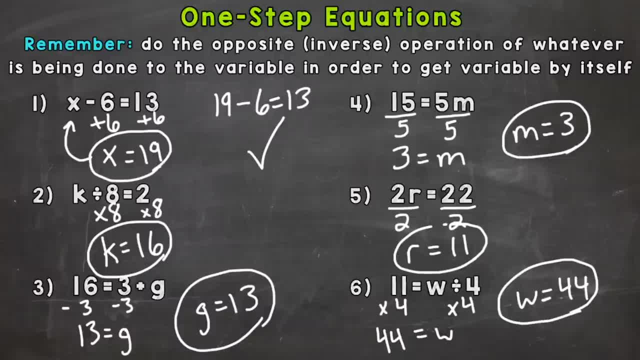 And let's double check. 44 divided by 4 does equal 11. So we're good to go with number six. So there you have it. There's how you solve one step equations. Hopefully you found that helpful. Until next time, peace. Bye. Bye. Bye. Bye. 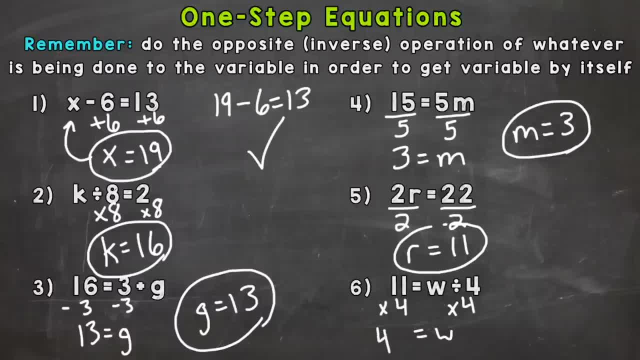 So we end up with an answer of 44.. 44 for the value of w, So w equals 44. And let's double check: 44 divided by 4 does equal 11.. So we're good to go with number 6..